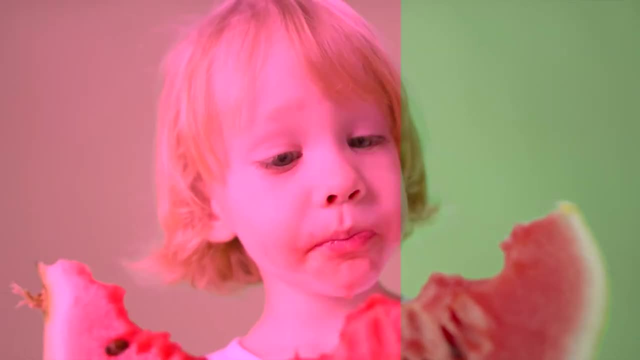 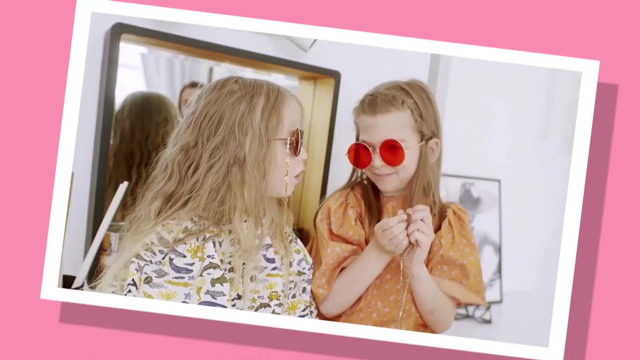 you don't have to be a grown-up to pursue photography or movie making. giving your child a camera can open their eyes to the world and provide you with insight on what it looks like from their perspective. the most important thing to consider is age. a kid prefers different gadgets at 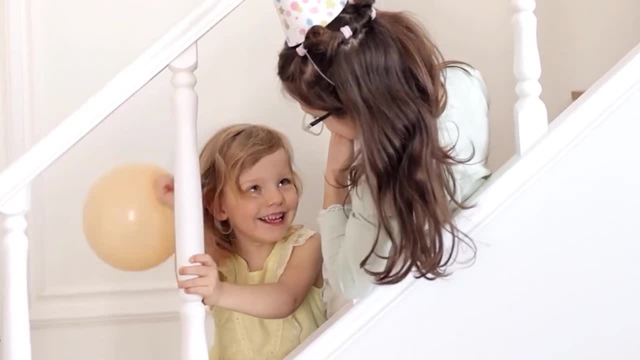 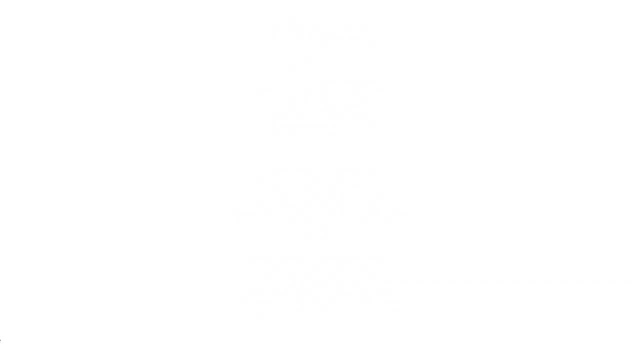 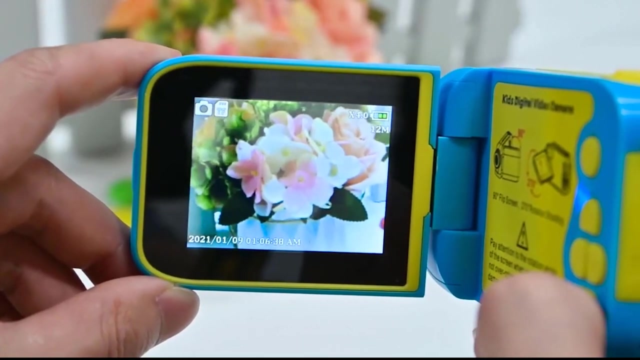 different ages. younger kids will enjoy shooting with easy to use and durable cameras. for them, photography is more like a game and cameras are like toys. luckily there are toy-like cameras that actually function and can take pictures, but later they can find the artistic and technical side of photography more interesting. they might care about video resolution, zoom range or even. 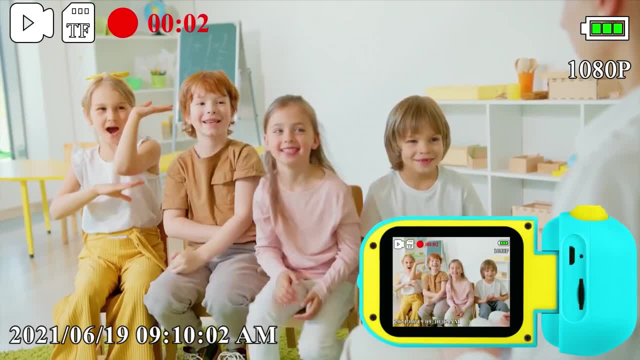 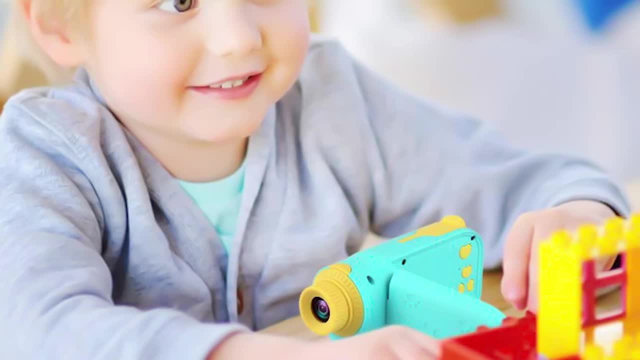 want to take, for example, time-lapse videos. choosing the best video camera for kids needs a lot of consideration, but no need to be worried. we've highlighted the three best choices for kids video cameras here. before i start reviewing, as always, i'm placing a link on each product. 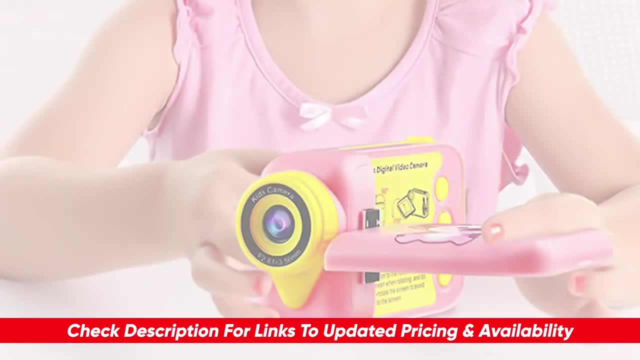 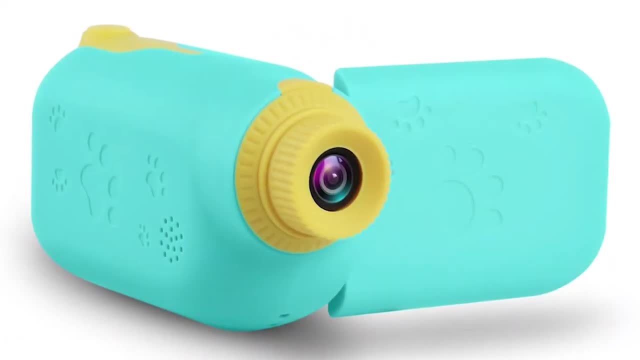 selection in the description of this video so you can check out the latest pricing and availability for any you might be interested in. also, if there are any special deals or discounts on each product, i'll include them in the description as well. well guys, i want to start. 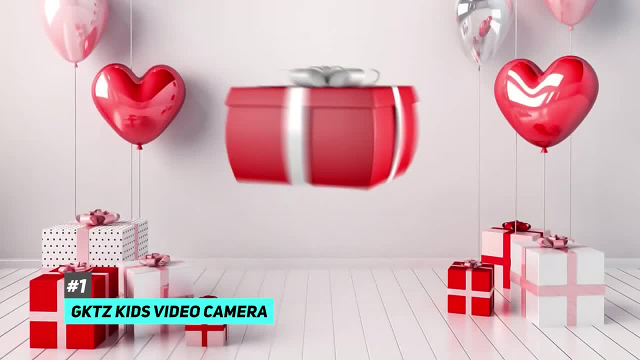 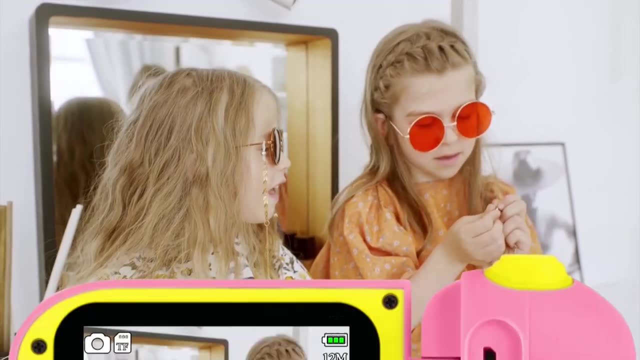 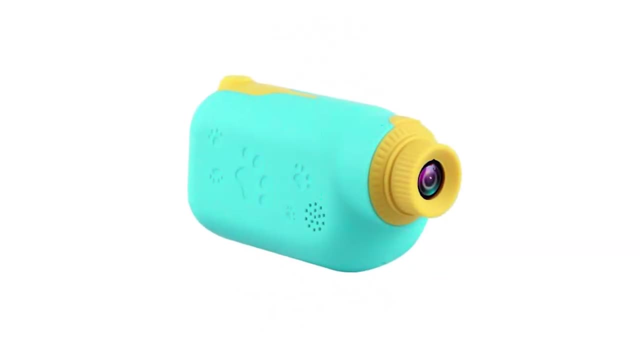 developing their creativity and imagination. the dimensions of this gktz kids video camera is 5.35 by 3.15 by 2.13 inches, with 3.35 ounces weight. this kids video camera has multiple functions, such as photo, video, voice recording and five different developmental games. speeding. 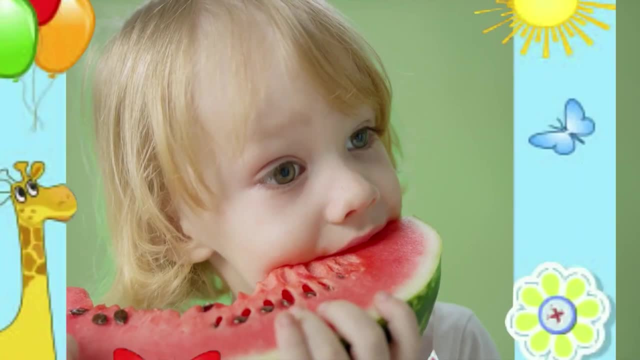 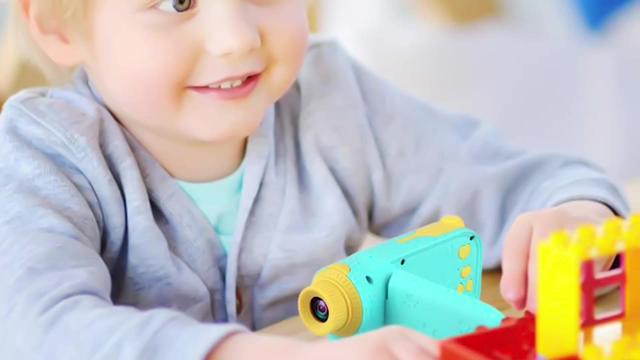 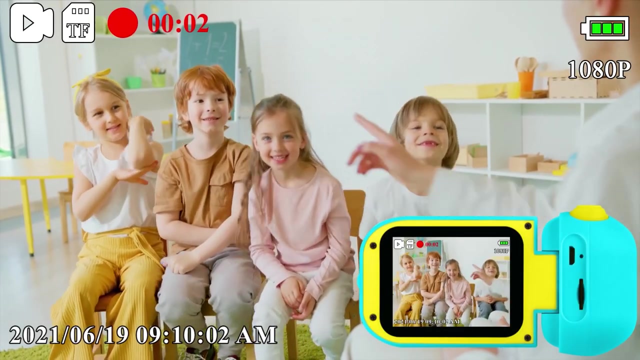 up the development of children's intelligence. there are funny effects on the kids video camera. the kids camera has built in 15 nice photo frames, three distorting mirror effects and six filter effects. children can choose their favorite effect before taking pictures. it's great for developing children's creativity and imagination. this kids video camera supports hd video resolution and max. 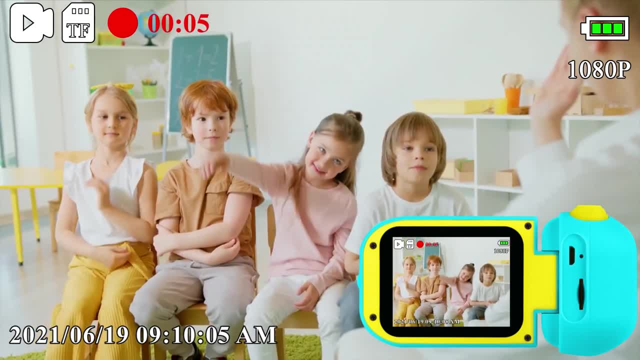 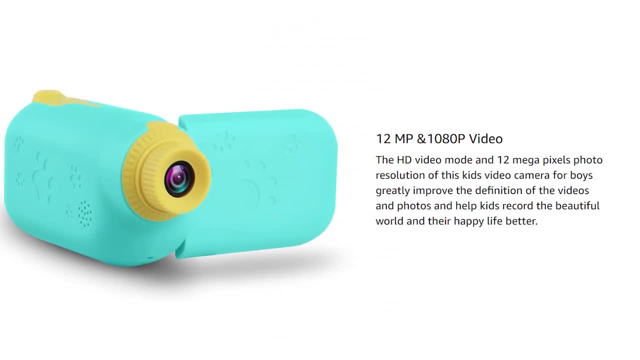 12 megapixel jpeg image resolution. the 2.4 inch ips touchscreen protects kids eyes. the four-time digital zoom-in function helps to capture clear scenes. the built-in rechargeable 800 milliamp battery enables kids to enjoy their photography time for about two to four hours. the gktz kids 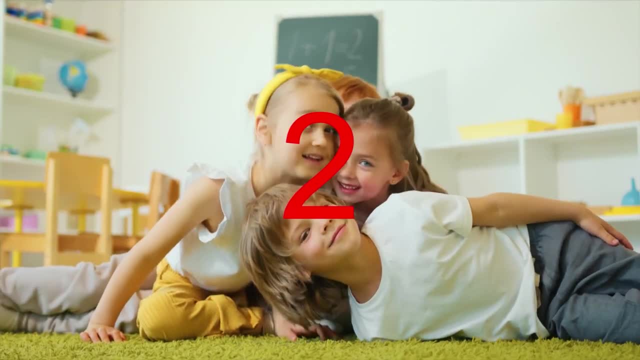 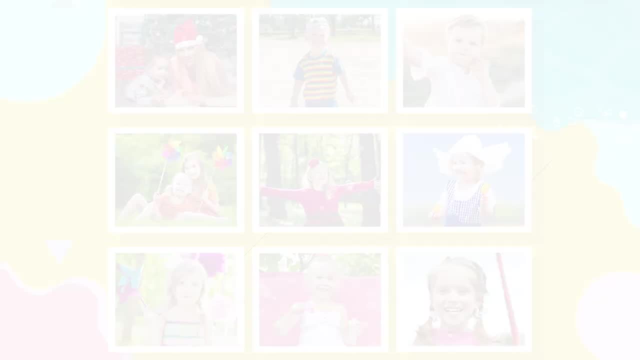 video camera supports time-lapse photos and burst mode. the timing function supports time-lapse taking photos in two second timing, five second timing and 10 second timing, and supports continuous shooting three at a time. the kids camera comes with a 32 gigabyte memory card. kids can insert the 32 gigabyte. 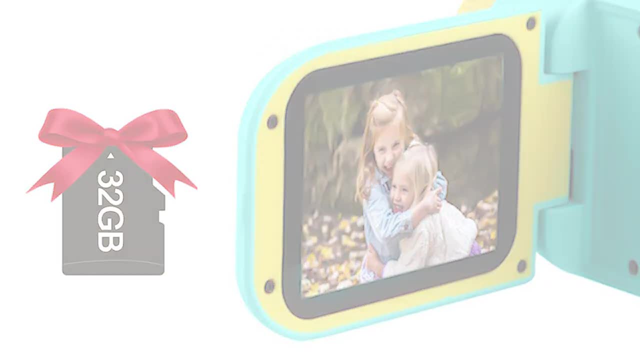 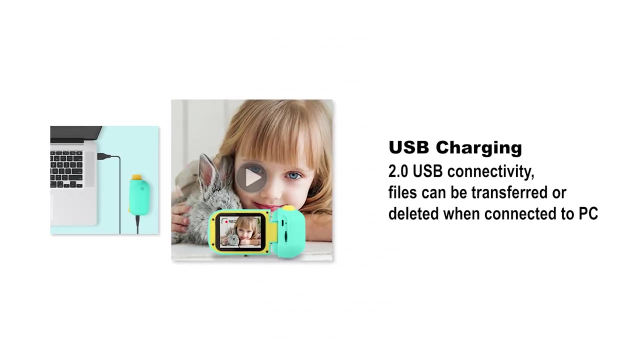 memory card to use this kids camera instantly taking pictures or videos. it can connect with the pc and desktop computer to charge by using the included 2.0 usb cable. you can also transfer all files to pc or delete files. when connected with the computer, it's easy to view and save the. 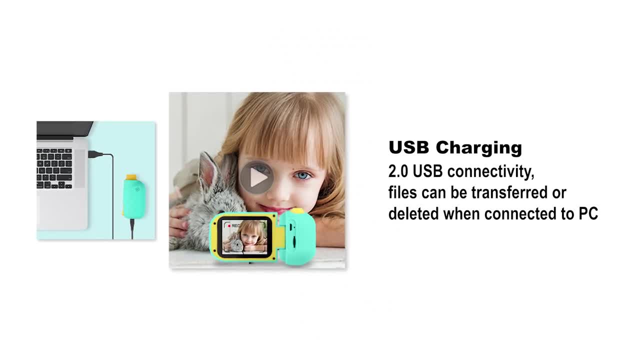 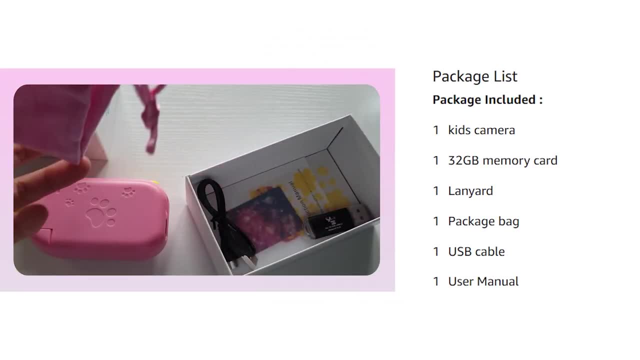 memories on camera, print beautiful photos and keep them forever. note: please: charge it with a 5 volt or charger, or connect the 2.0 usb port to charge what you get in the package: one kids camera, 132 gigabyte memory card, one lanyard, one package bag, one usb cable and one user manual gktz kids. 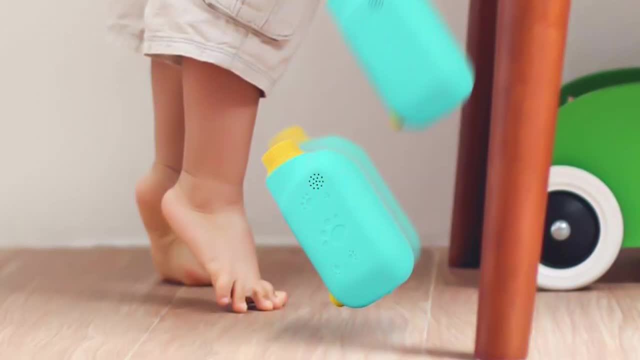 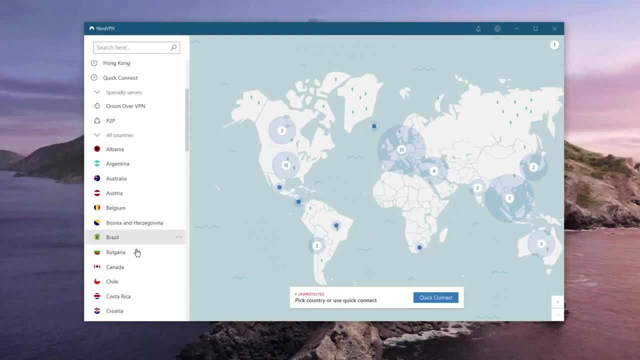 video camera is made of high grade material. it's shock proof, safe design and skin comfortable for kids. it comes with a carrying bag and hand lanyard easy for carrying the mini kids video camera to everywhere. by the way, today's sponsor is nordvpn. they're consistently the top choice for staying. 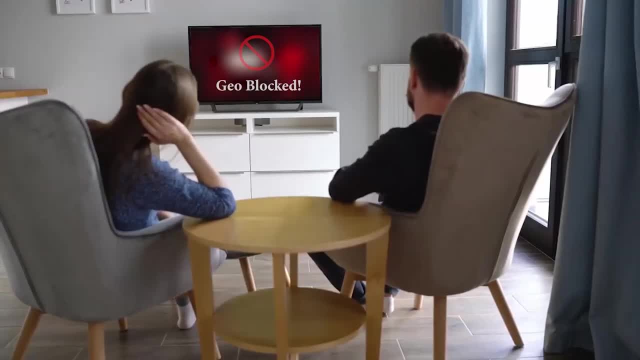 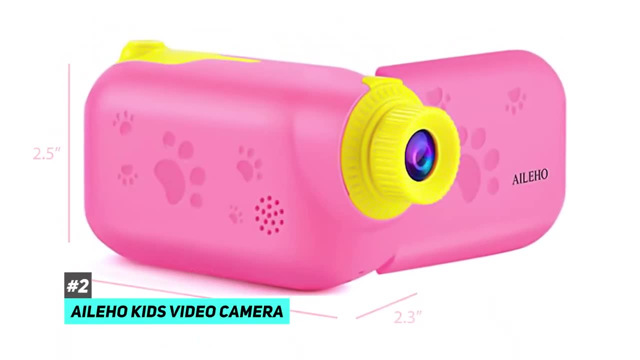 anonymous online, torrenting safely and accessing geo-restricted streaming content. you can check the description for a full review, along with a special discount, if interested. the second best three is alejo kids video camera. the dimensions of this kids video camera is 4.5 by 2.5 by 2.3 inches and 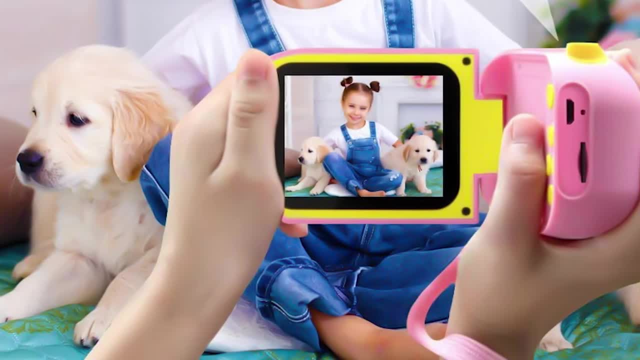 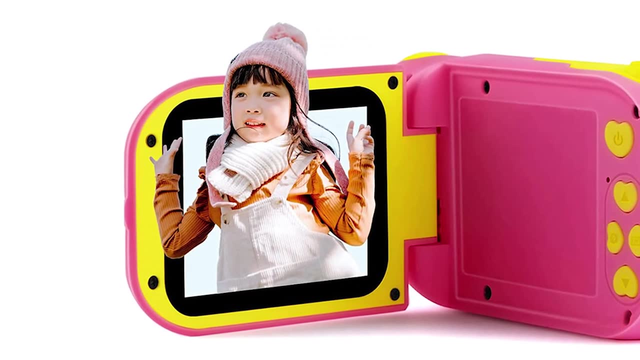 3.29 ounces weight. the alejo kids video camera is equipped with 1080p high resolution video, hd ips screen, fhd video resolution. the supersized screen protects kids eyes by high definition of the pictures and videos. take excellent videos. kids will capture the happiness time with family. 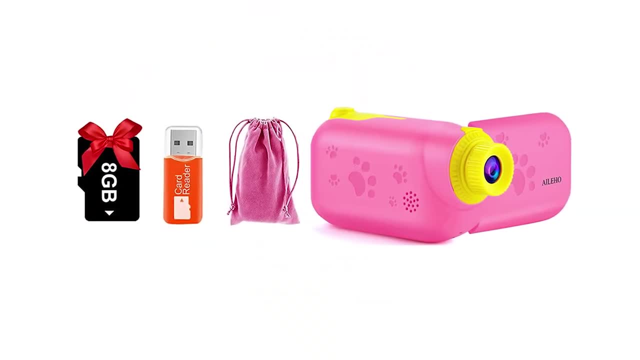 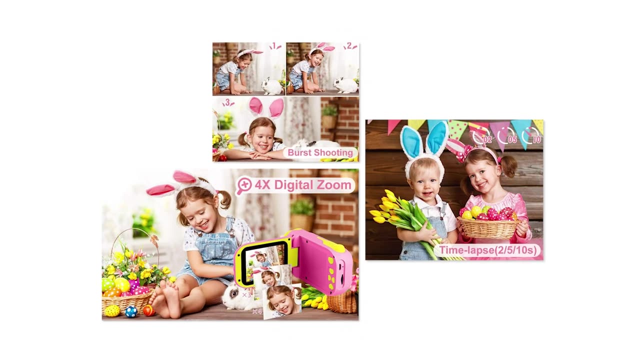 members and friends with their kids camcorder, gifted with an eight gigabyte tfp camera. the kids card enables kids to take pictures on unboxing. the kids video camera supports 12 megapixel and four-time digital zoom. a good start camera for kids to learn about photography. this children's 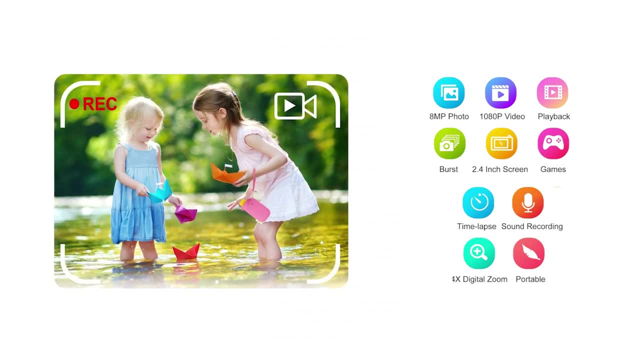 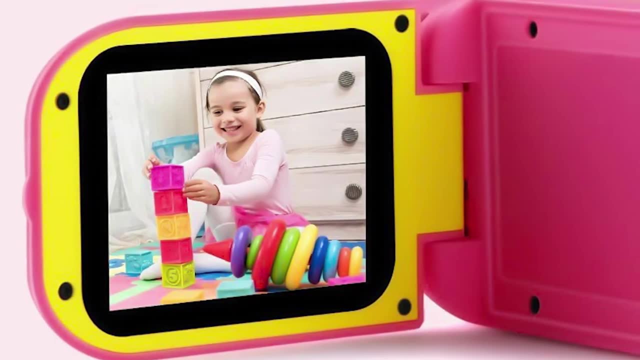 video camera can also stimulate kids creativity and imagination, cultivate their hobbies in photography and exercise their physical coordination. it's very suitable as a video camera for kids to capture every moment and make their own youtube videos. this digital camera for kids comes with 15 lovely frames, six different filters, three pranking special effects and five. 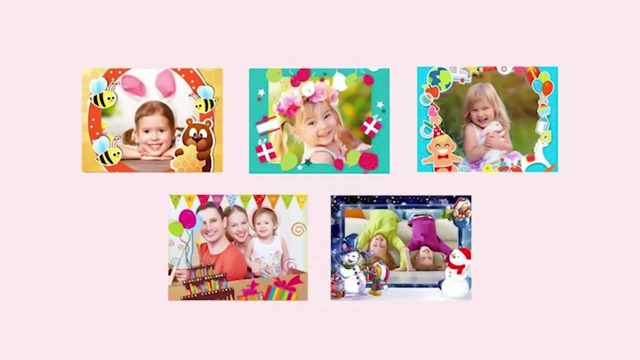 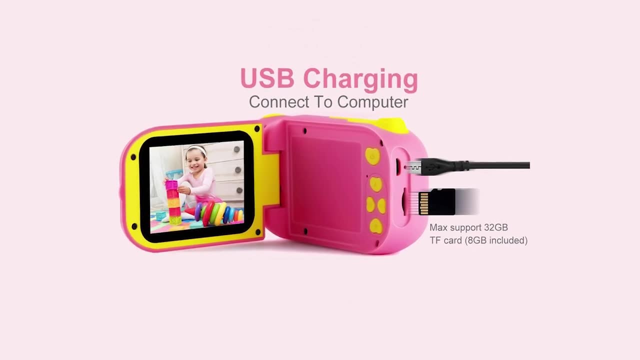 puzzle games. kids can choose their preferable frames or special effects. capture the moment in nature and enjoy photography with their own ideas. download photos and videos to a computer using the included micro usb cable and share them with family and friends. this kids camcorder is equipped with a large battery of 1000 milliamp. toddlers can play with the alejo kids. 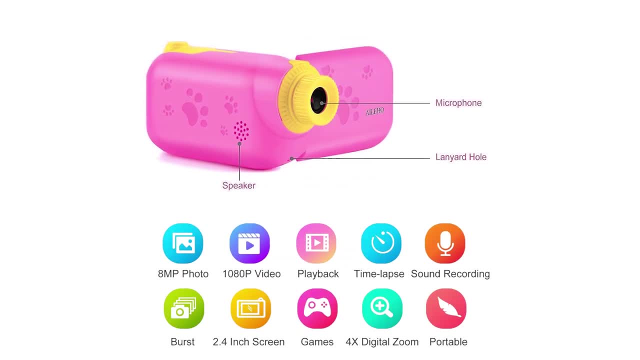 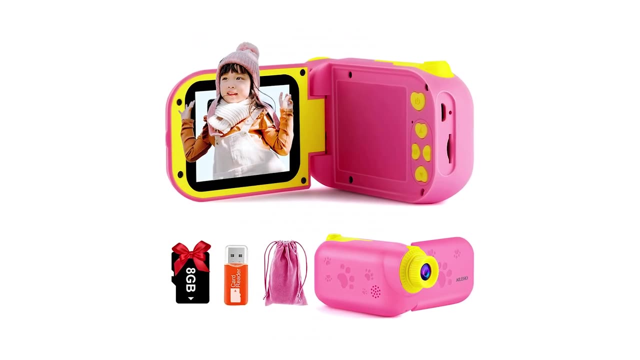 camera for two to three hours after fully charging. this children's camera has time lapse, burst, playback, sound recording games, 13 language options, date stamp on pictures. what you get in the package: one kids camera, one 32 gigabyte memory card, one lanyard, one package bag, one usb cable, one user. 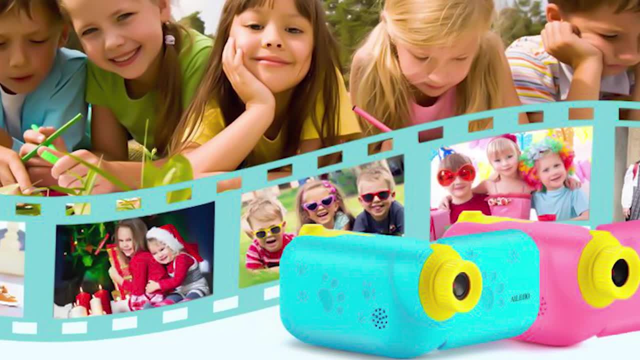 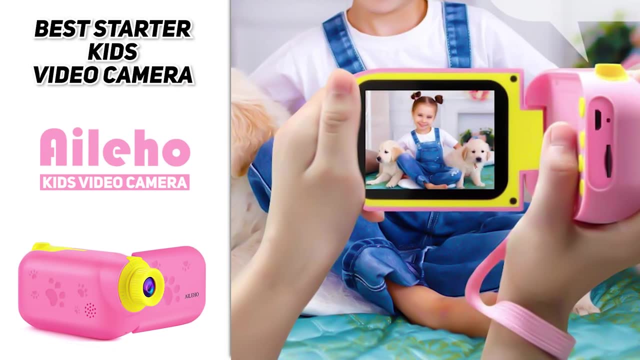 this kids video recorder is gifted with a carrying bag and slings, so this camera for children is portable to be taken along with kids to anywhere. this kids video camera is the best choice as a birthday holiday gift for three to nine year old children. last but not least is the pro grace kids. 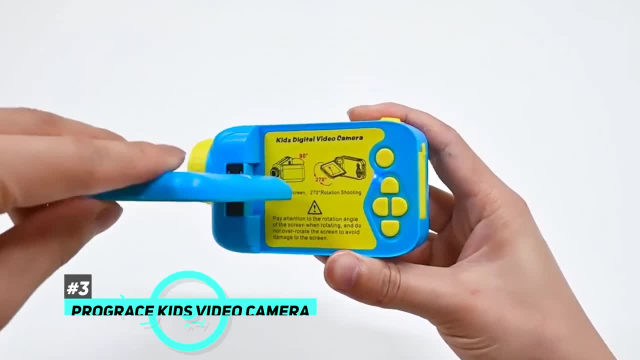 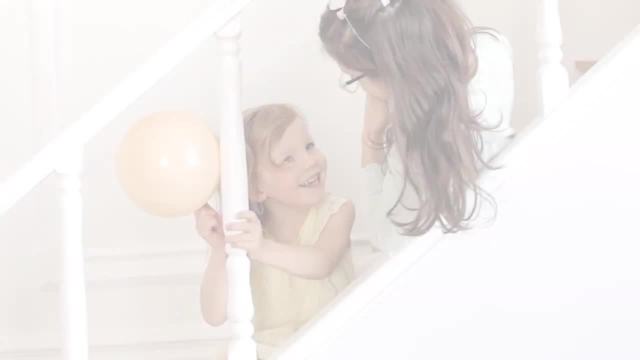 video camera. this pro grace has 270 degree rotatable video camera. the 2.4 inch display can be rotated in four different directions, allowing you to take pictures from various angles. this video camera is equipped with 12 megapixel photo and 1080p high resolution video. 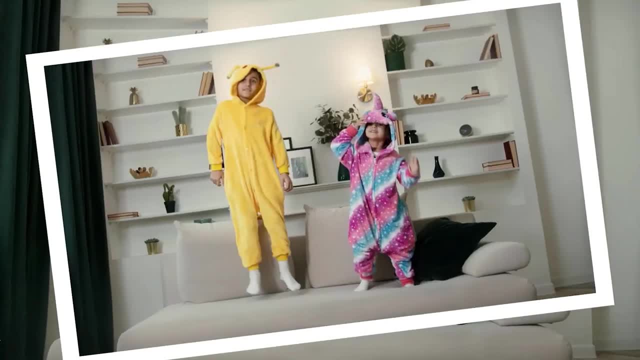 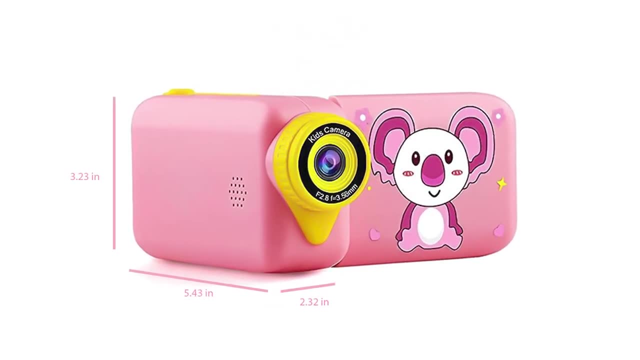 kids can use this camera to take hd pictures or videos. supports taking selfies and recording voices. kids will love their own cute camera. the dimension of this pro grace video camera is 5.43 by 3.23 by 2.32 inches. with 7 ounces weight, this kids digital video recorder can 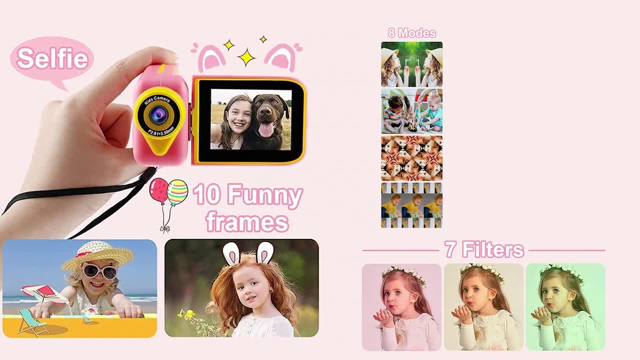 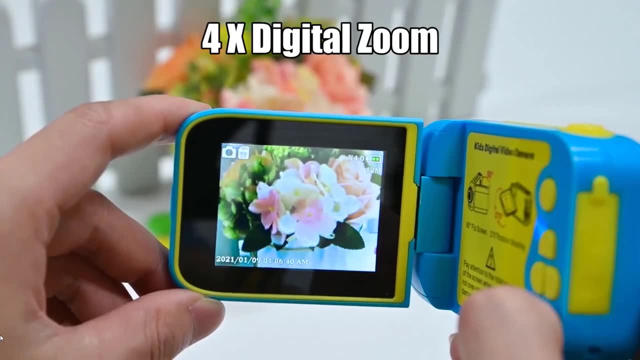 take unique sketch photos. it has 10 funny photo frames, 8 prank special effects for children to choose from. built-in four-time digital zoom, continuous shooting and time-lapse shooting. children will enjoy the interesting photo effects they get. this kids camera camcorder is built in. 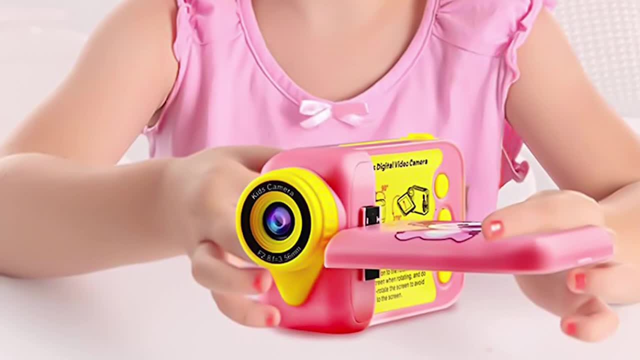 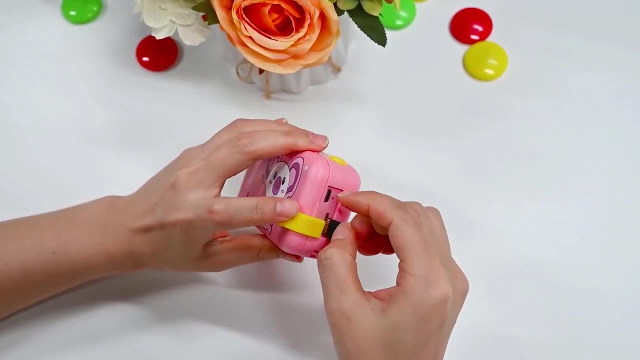 capacity: 1000 milliamp rechargeable battery which can take photos for three to four hours. it comes with a usb cable and can be charged with a 5 volt 1 to 2 amp adapter. it also comes with a 32 gigabyte micro sd card that can store more than thousands of photos. what you get in one package. 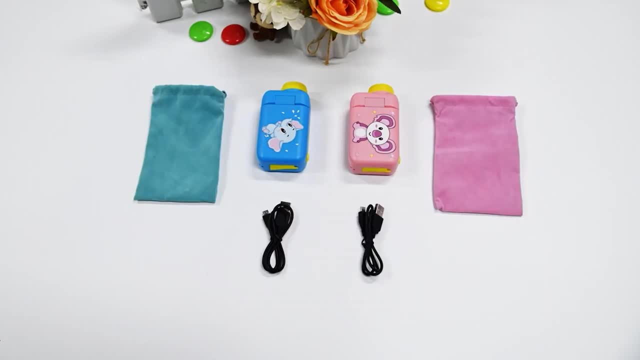 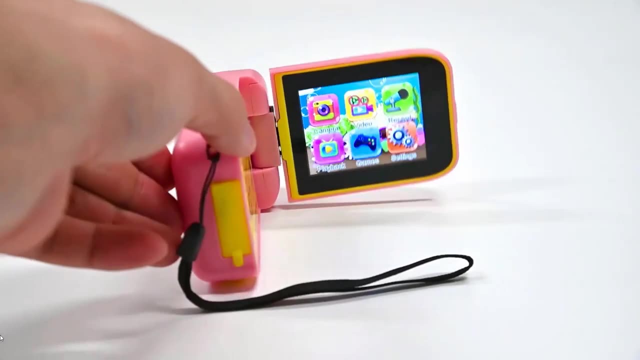 one rotatable camera for children, one 32 gigabyte micro sd card, one usb cable, one flannelette bag, one lanyard, one user manual. this kids video camera is made of high quality, non-toxic material. it's safe and comfortable. this toy camera comes with a lanyard and camera.